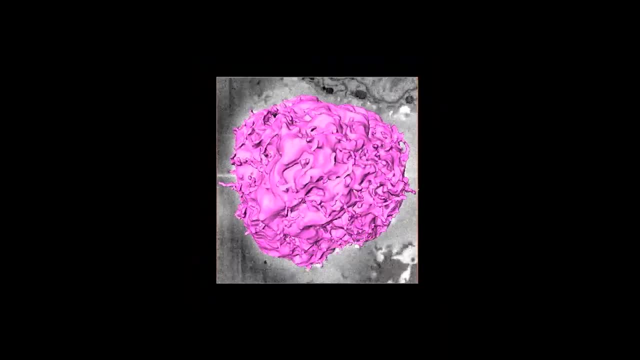 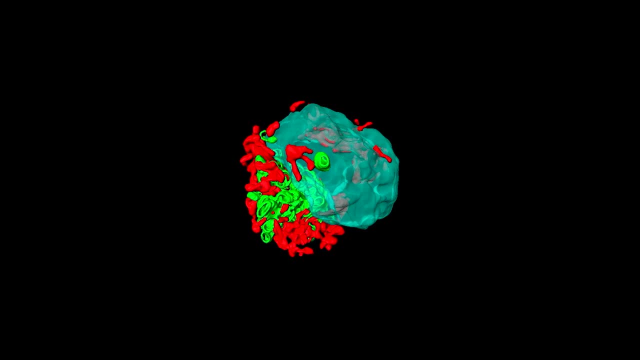 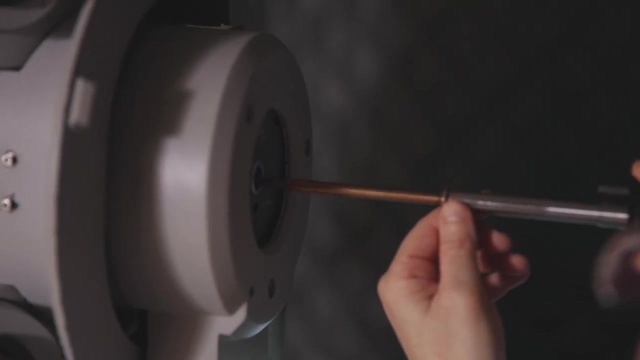 We found that these lysosomes were surrounded by the mitochondria at one pole of the cell and the whole exchange of the iron is going from the lysosomes to the mitochondria where heme is produced. And basically it was just a beautiful study of structure function relationship, which 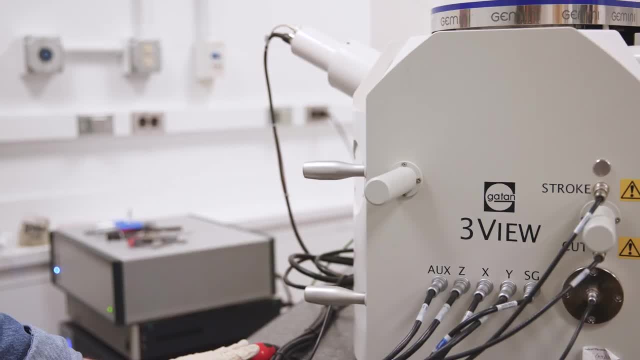 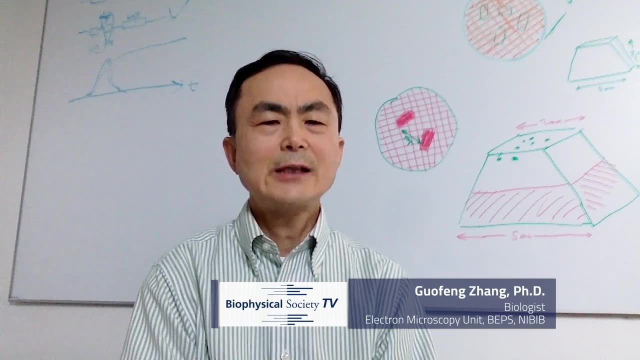 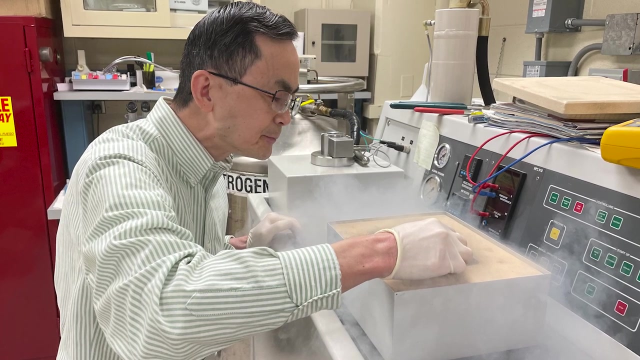 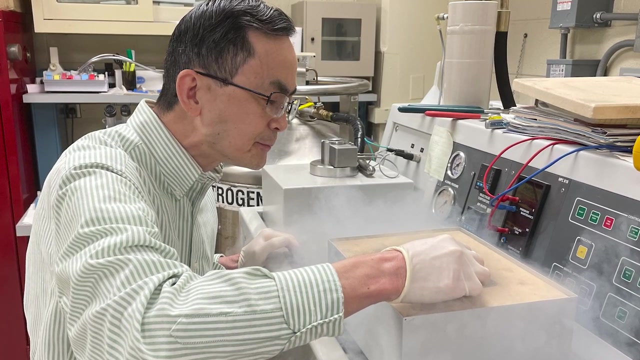 you need to do in three dimensions because you can't tell what happens in 2D. The 3D electron microscope in our lab relies on using fixatives together with heavy metals to staining cells and tissues that are embedded in plastic. Sometimes we also use high-pressure freezing method to preserve the ultra-structure for 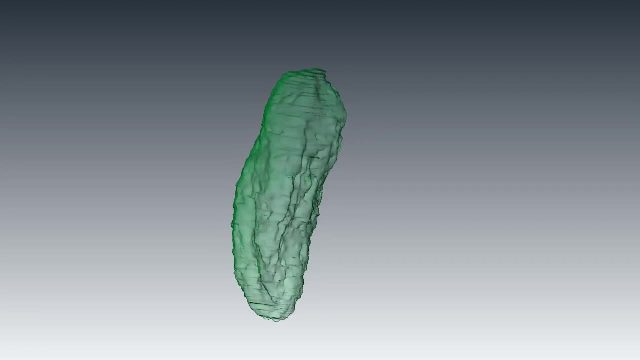 high-resolution studies. We've been working recently on platelets, and in doing this we have a joint collaboration then with the US Department of Health and Human Services. We've been working recently on platelets, and in doing this we have a joint collaboration then with the. 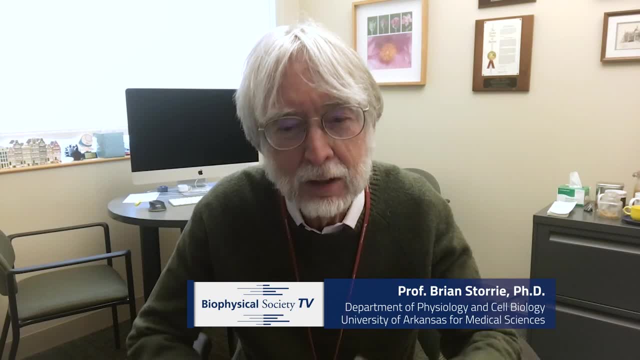 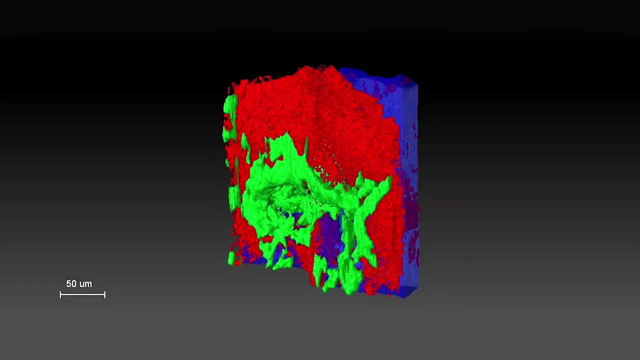 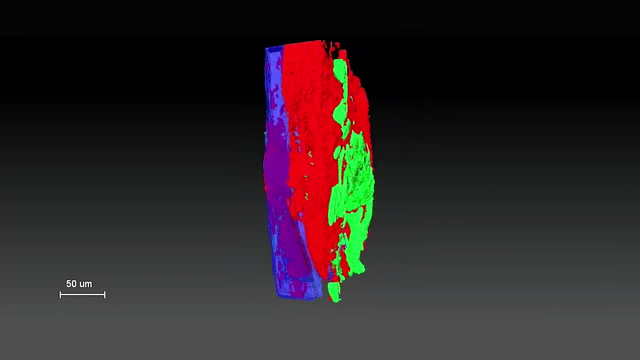 Richard Liebman's lab at the NIH and with the advances in 3D volume imaging, using new technology we were able to image the entire thrombus that forms. that is, the platelet aggregate that actually stops bleeding, and we were able to do that in 3D and we've moved. 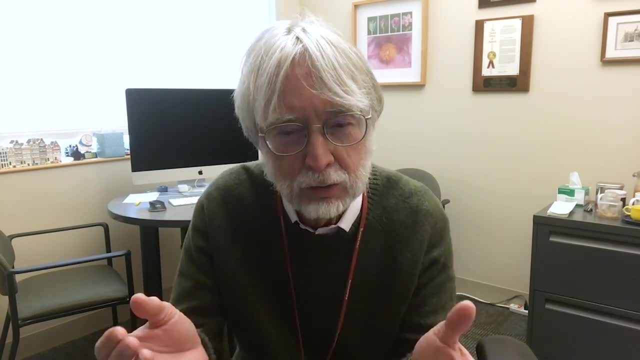 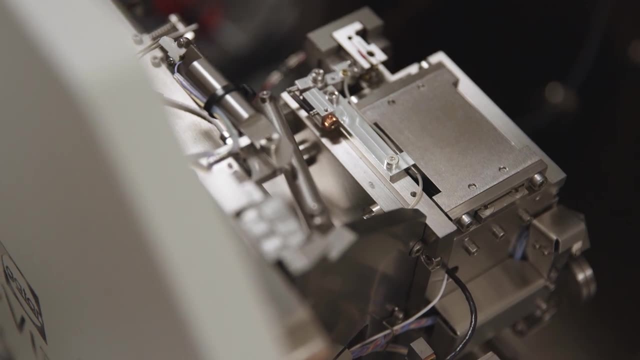 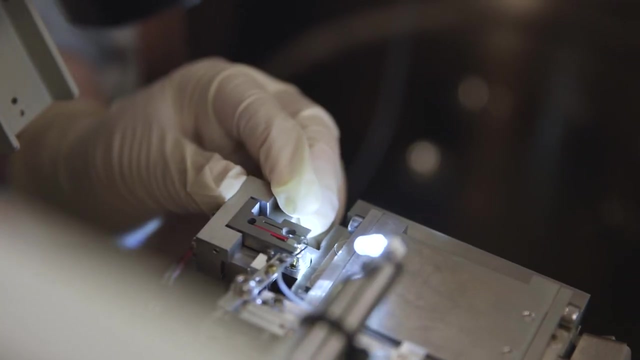 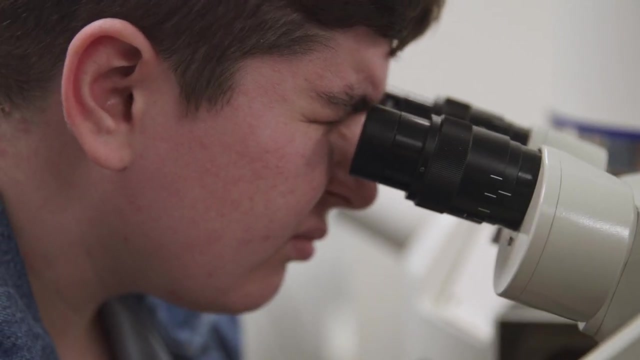 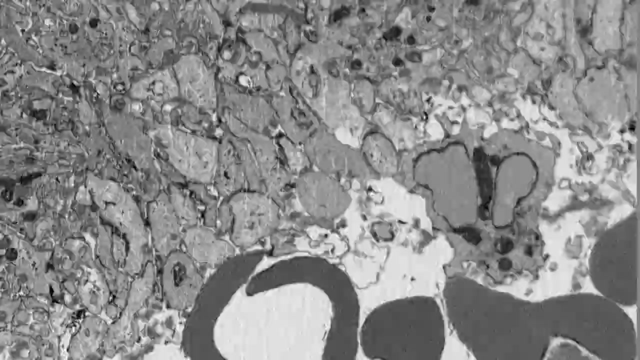 on now to trying to handle the problem of occlusive clots, those things which form in arteries and what are the real risk factors in terms of stroke or myocarditis. There's two projects our lab is working on that I'm a part of. The first is a project with COVID blood samples, and the other project that we're working on is on occlusive blood clots and examining the structure of the blood clot, as to where red blood cells are within it, how tightly packed the platelets are, and so on. 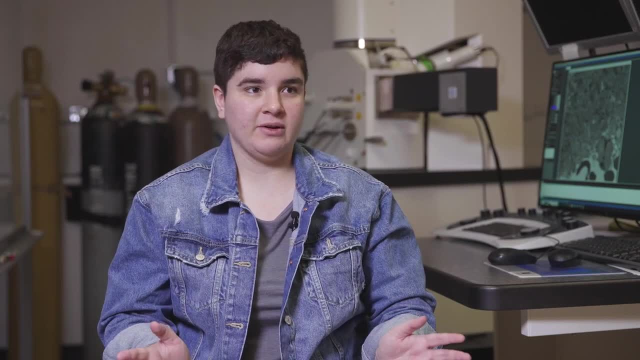 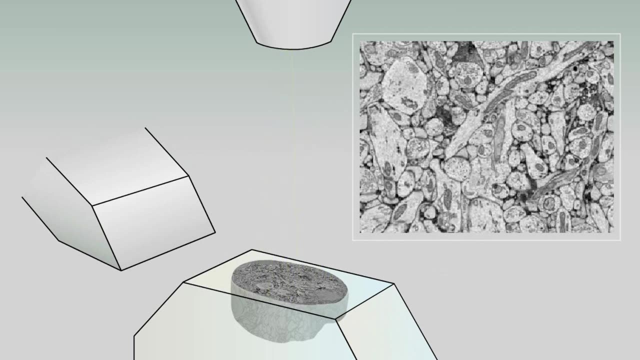 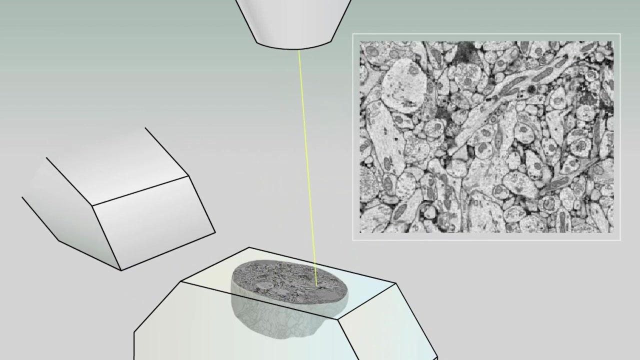 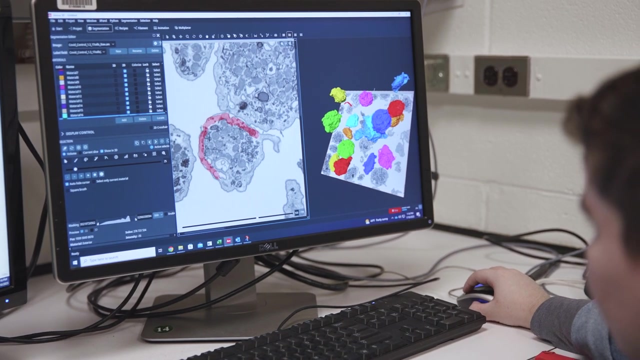 The serial block face. SEM is one of the techniques that we're working on. It essentially just images a sample and then with a tiny diamond blade it scrapes off a layer, images the layer underneath and keeps doing that until we get a 3D representation of our sample. and then we take that over to our software, where we analyze the data and we segment it and are able to generate 3D models.